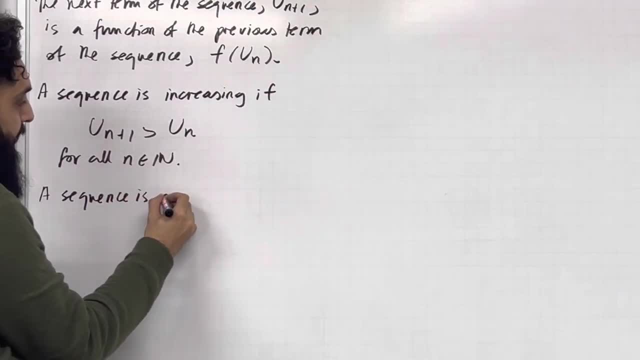 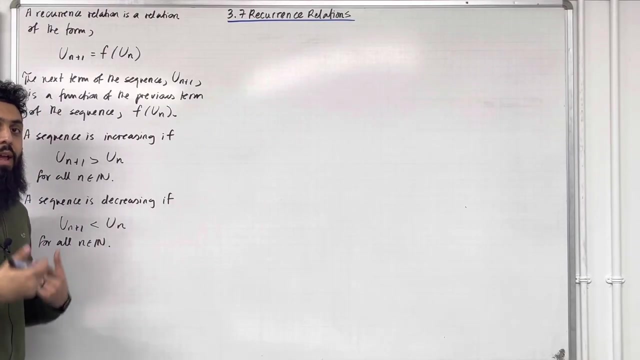 A sequence is decreasing if un plus 1 is less than un for all natural numbers n. Now we're going to look at a periodic sequence, For example 1, 4, 7,, 1, 4, 7, and so on. 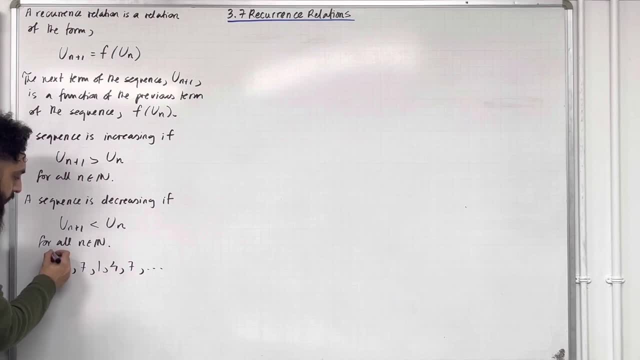 Now over here, what we notice is that there's a repetition in cycles of 3. We call this a periodic sequence, Periodic sequence, And that repetition is called the order of the sequence. So in this case, the order. 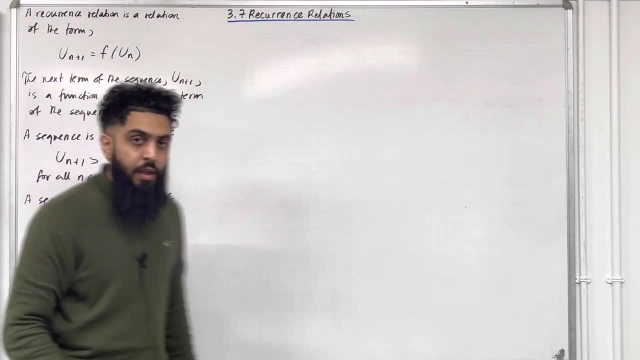 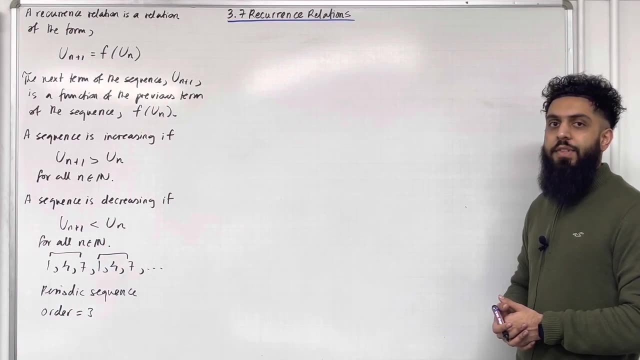 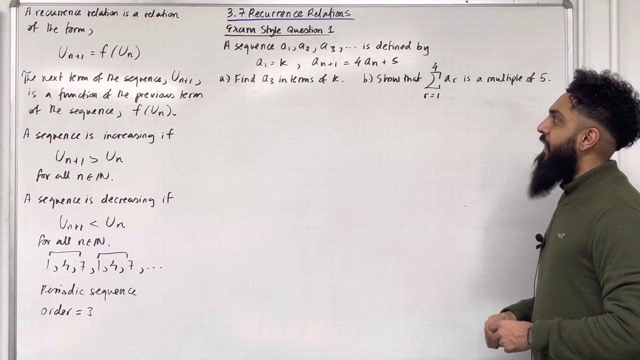 Is equal 3.. So, ladies and gents, these are all the key facts of 3.7, recurrence relations. I'll be implementing these key facts within exam style questions. Here's exam style question: 1.. A sequence- a1,, a2,, a3,, dot, dot, dot- is defined by 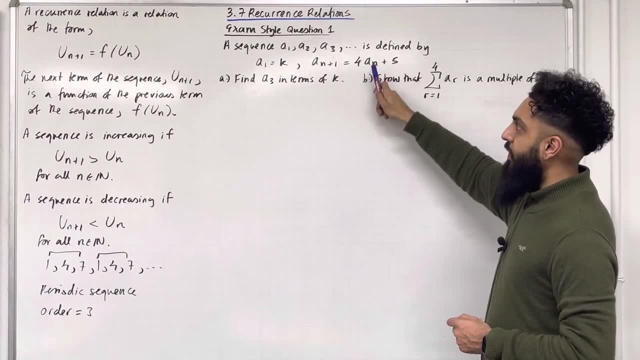 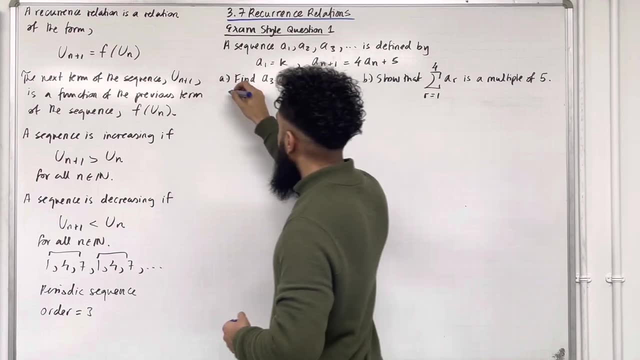 a1 is equal to k. an plus 1 is equal to 4, lots of an plus 5.. Part A find a3 in terms of k. Ladies and gents, we know that a1 is equal to k, n plus 1 is equal to 4, lots of n plus 5.. 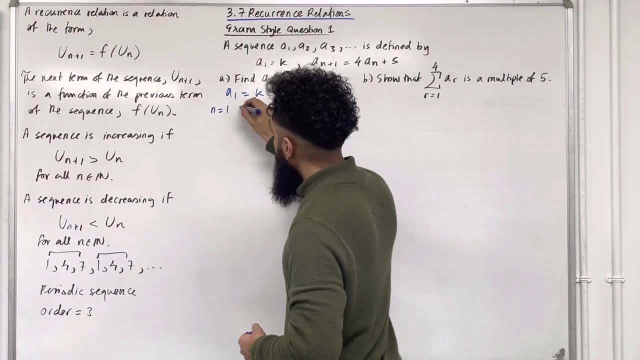 Ladies and gents, we know that a1 is equal to k, n plus 1 is equal to 4. lots of n plus 5. k- We can substitute n equal 1 into here to work out a2. So we've got: a2 is equal 4, lots of a1 plus. 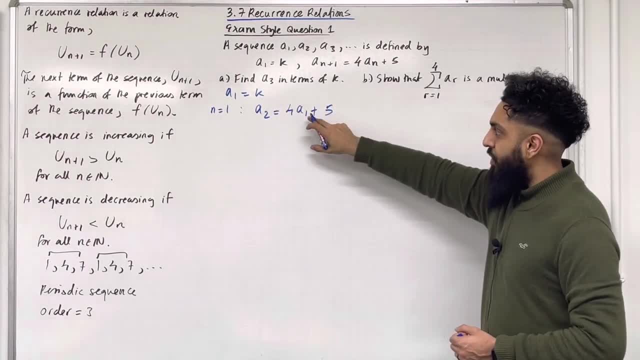 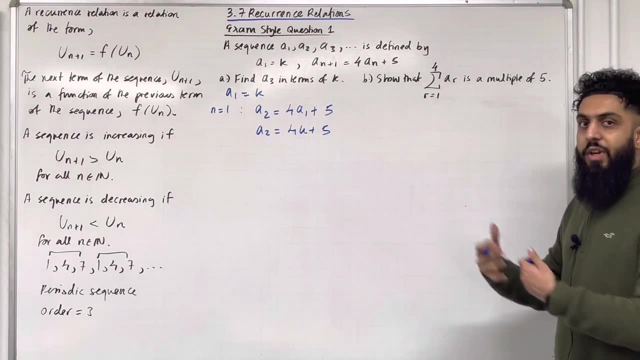 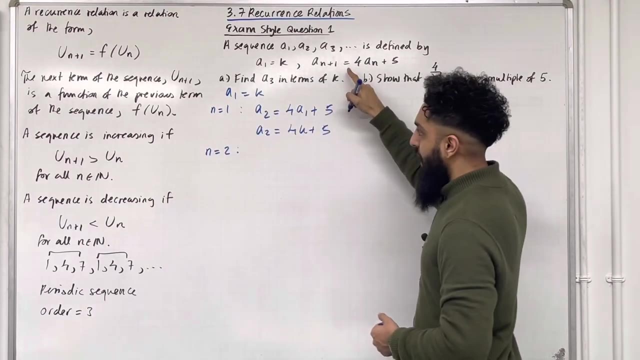 5. a1 is equal to k. we can substitute that into here. So we've got: a2 is equal 4k plus 5.. Now we can proceed forward and work out a3.. We can substitute n equal 2 into here to work out a3. 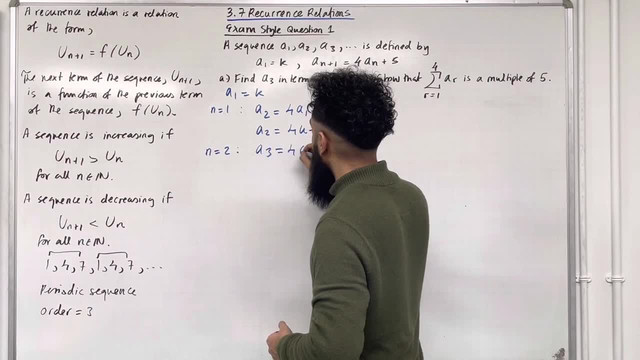 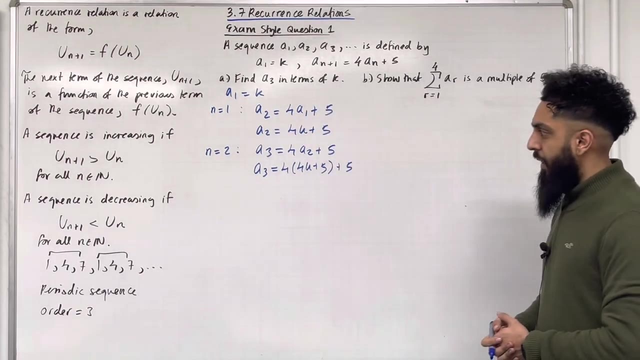 So we've got: a3 is equal 4- lots of a2 plus 5.. a2 is 4k plus 5, we can substitute that into here. So a3 is equal 4- lots of 4k plus 5, plus 5 outside the bracket. We can simplify this. 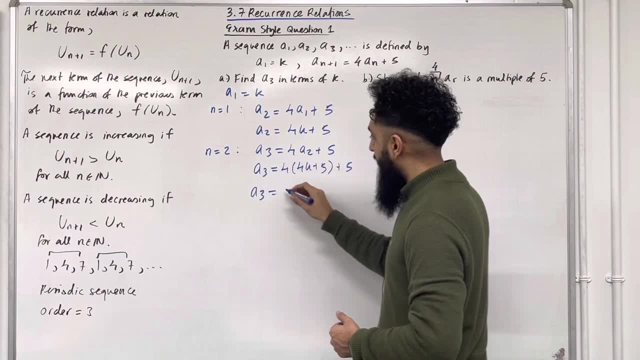 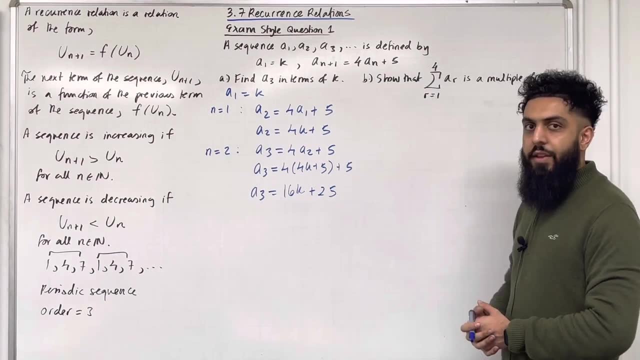 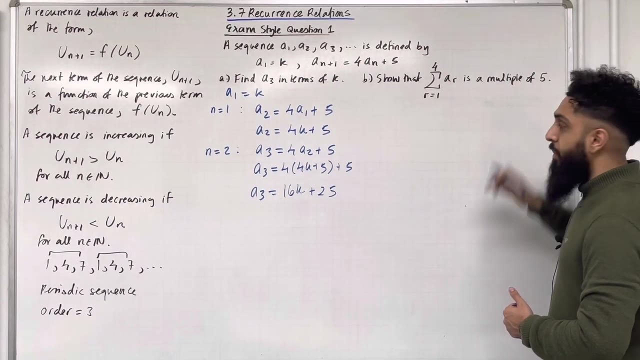 So we've got a3 is equal 16k plus 20 plus the 5, so plus 25.. That there, That is my a3.. Let's move on to part b. Show that the sum from r equal 1 to 4 of ar is a multiple of. 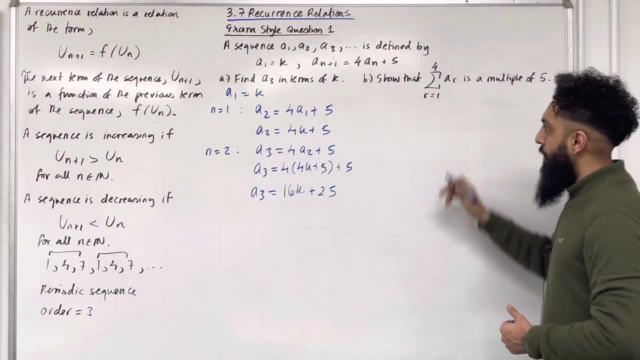 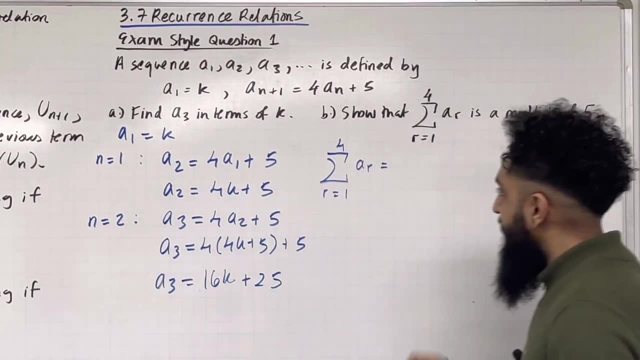 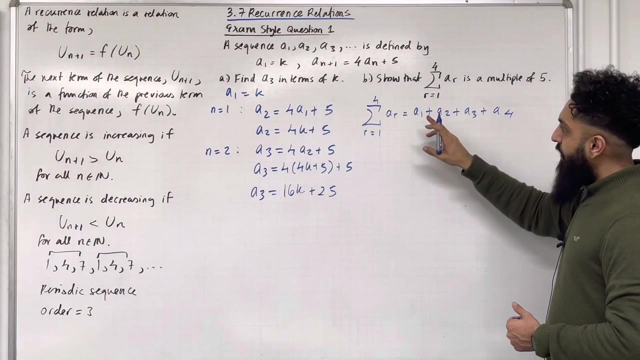 5. Ladies and gents, we can open up this sum. So we've got the sum from r equal 1 to 4 of ar. This is equal to a1 plus a2 plus a3 plus a4.. Now we already have a1, a2, a3, but what we don't have? 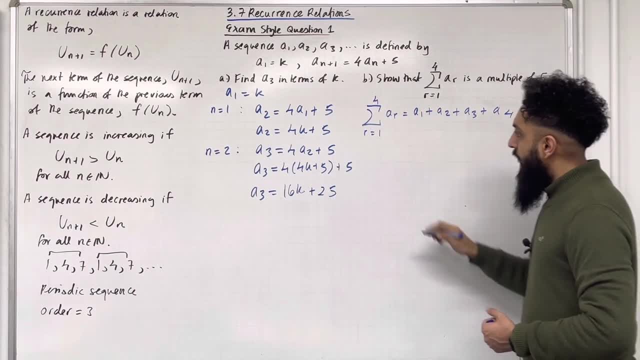 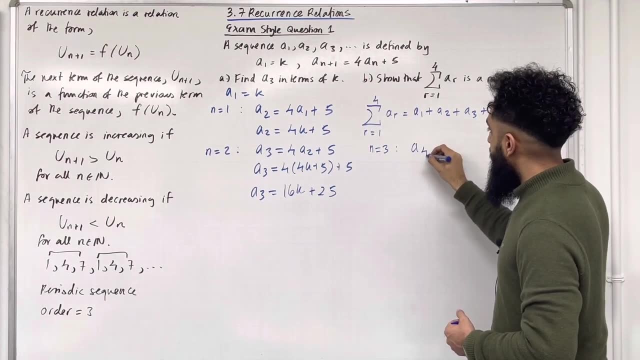 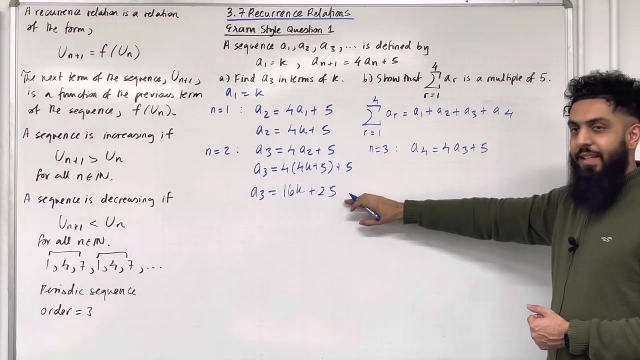 is a4. So we're going to calculate a4. I can substitute n equal 3 into here to work out a4. So I've got a4 is equal 4, lots of a3 plus 5.. I've calculated a3, which is 16k plus 25. I can substitute that. 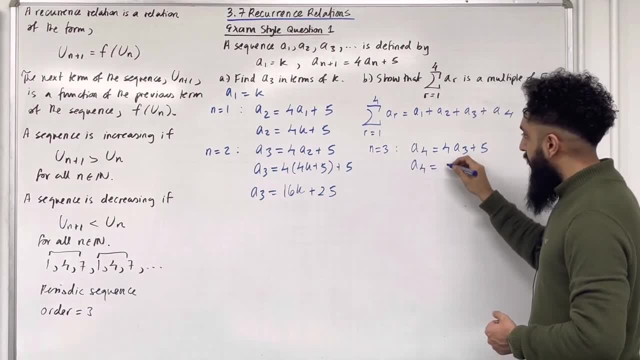 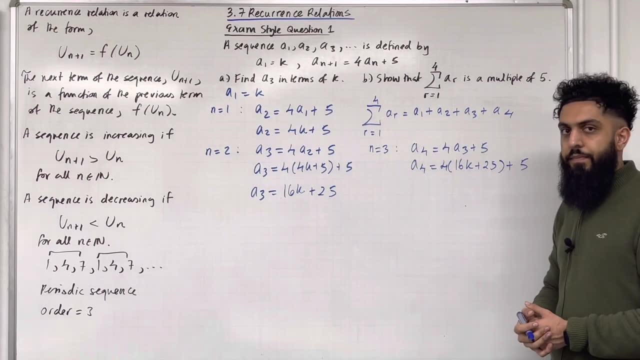 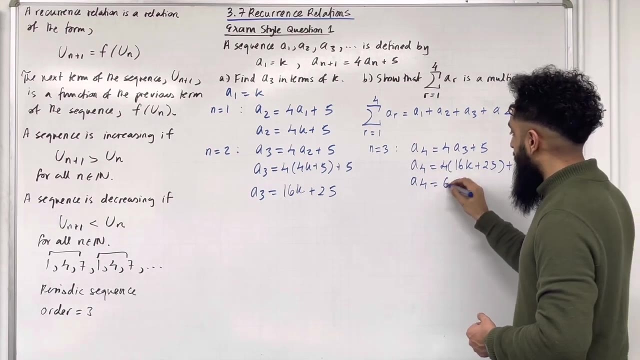 into here. So a4 is equal 4 lots of 16k plus 25 plus 5 outside the bracket, I can expand it. I can substitute that into here. So I've got a4 is equal 4 times 16k, which is 64k plus 4 times 25.. That's. 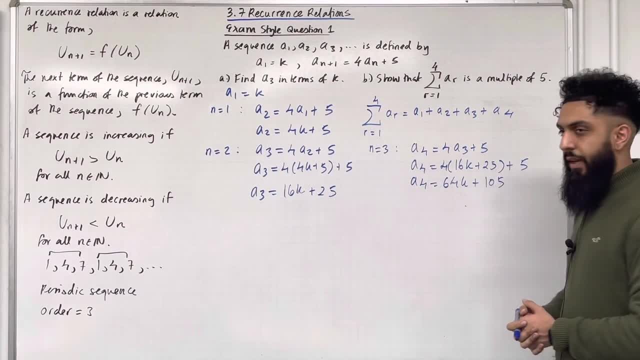 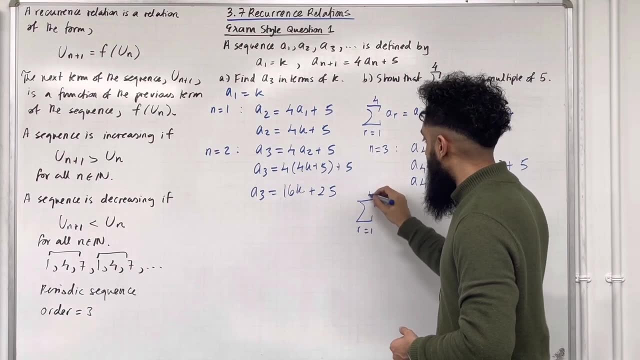 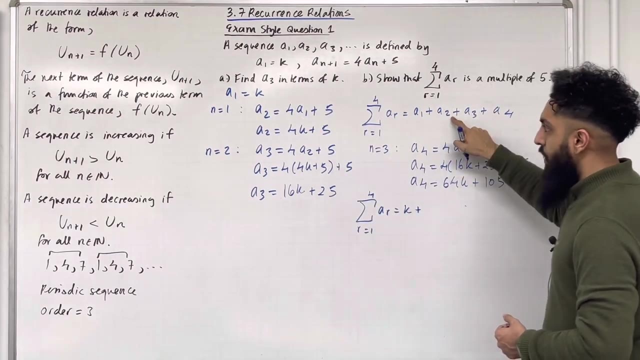 100 plus 5.. That's 105.. Now, ladies and gents, this sum over here, sum from r, equal 1 to 4 of ar, is equal a1, which is k plus a2, which is 4k plus 5.. 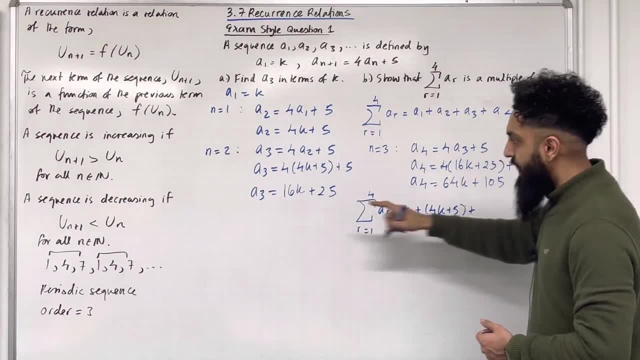 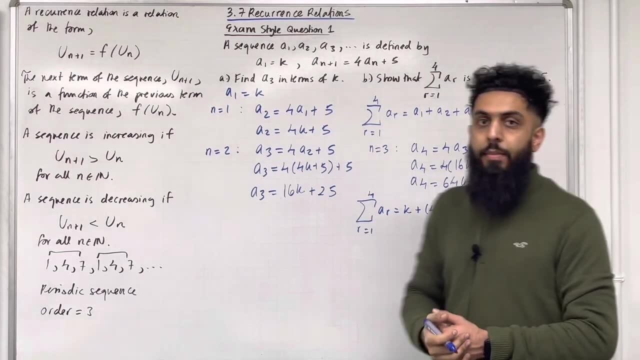 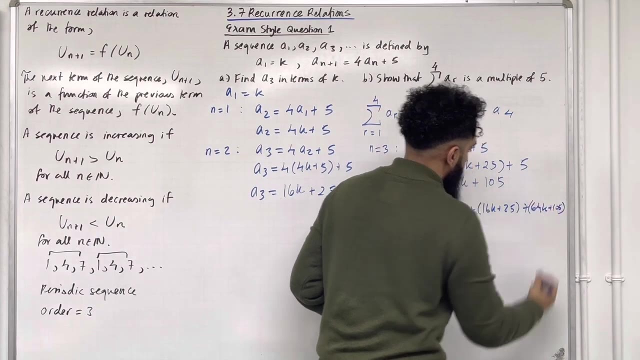 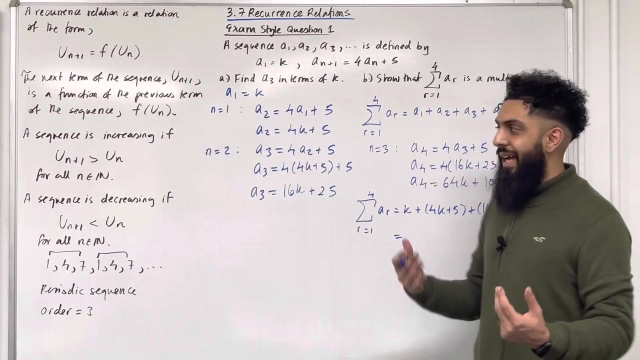 So I've got a4 plus a3, which is 16k plus 25, plus a4, which is 64k plus 105. So we've got 64k plus 105. Now we can add this together. We can simplify the expression, collecting the like terms and adding. 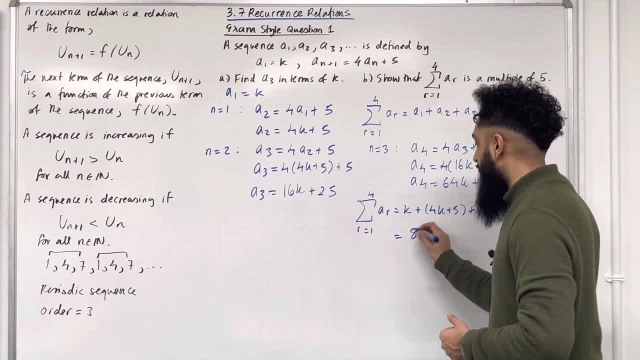 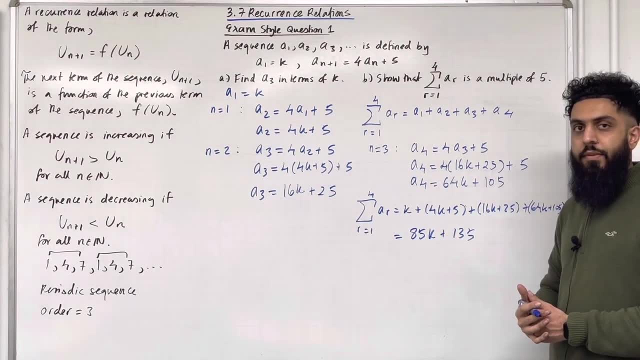 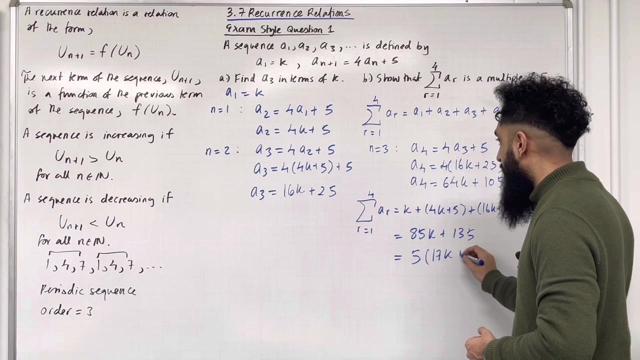 the constants. So if we add this together, we get 85k plus 105.. We want to show that this here is a multiple of 5.. We can take out a factor of 5.. So if we take out a factor of 5 inside the bracket, we've got 17k plus 27.. And, as you can see, this is a multiple. 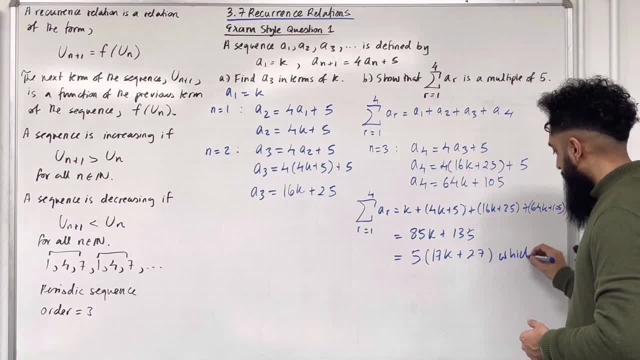 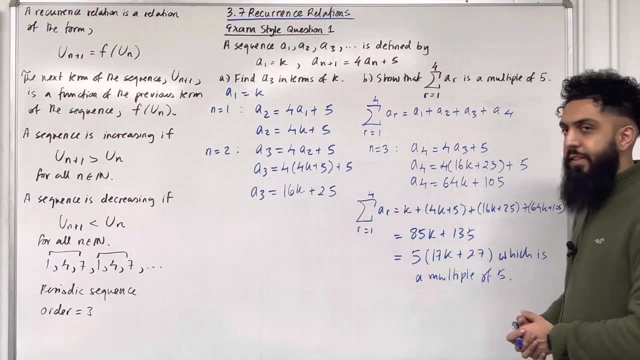 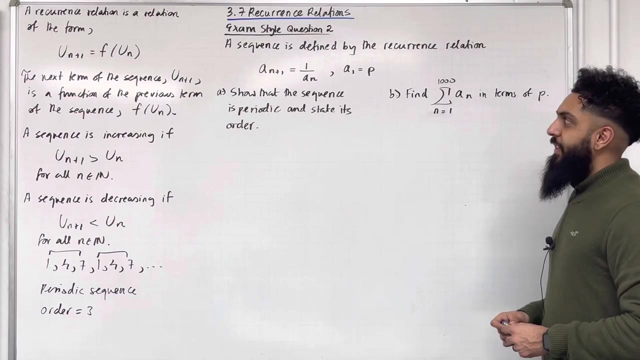 of 5, which is a multiple of 5, as required. This completes exam style, So we can start with the question 1.. Here is exam style question 2.. A sequence is defined by the recurrence relation. a n plus 1 is equal 1 over a n where a1 is equal. 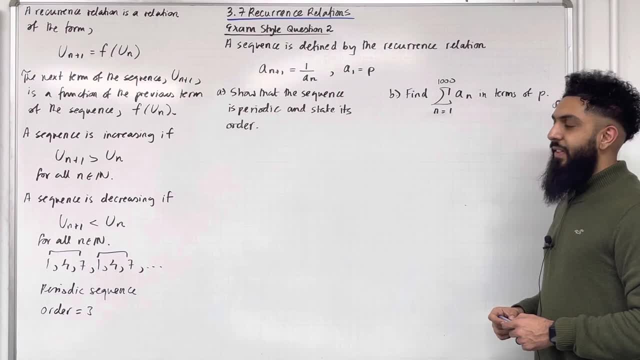 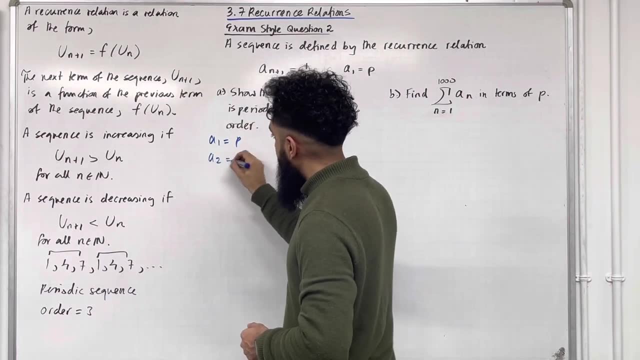 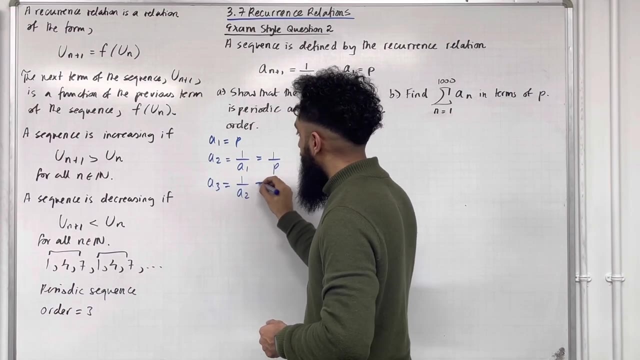 p Part a. show that the sequence is periodic and state its order. Ladies and gents, we know that a1 is equal p. a2 is equal 1 over a1. So that's 1 over p. a3 is equal 1 over a2.. So that's 1 over. 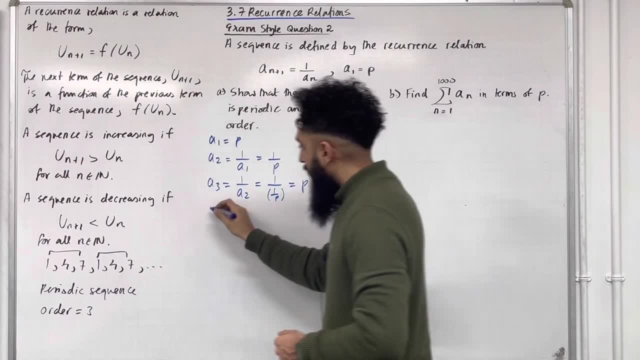 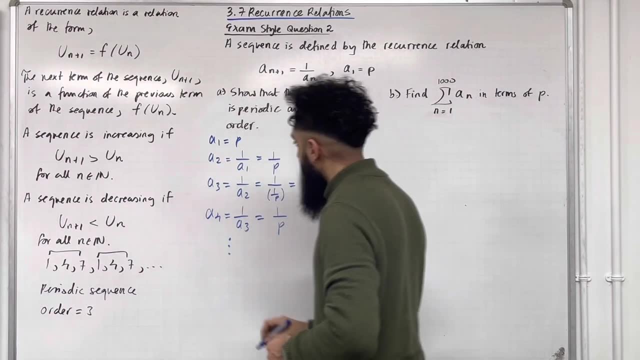 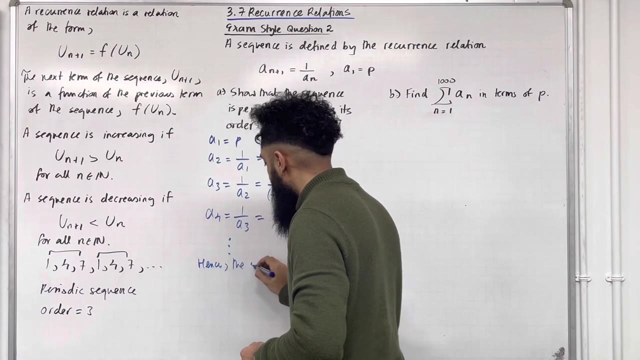 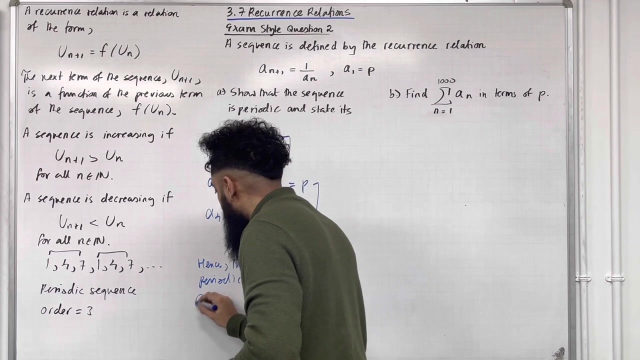 1 over p. This is just p. a4 is equal 1 over a3.. So that's 1 over p. Dot dot dot. We have a repetition in cycles of 2. Hence the sequence is periodic And the order of the sequence is 2. 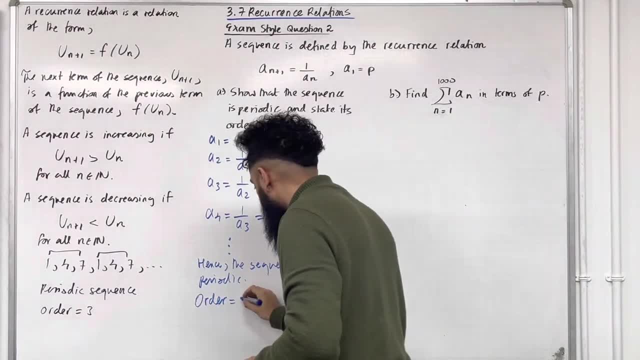 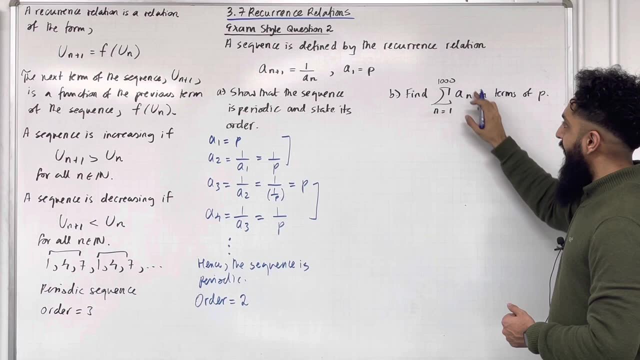 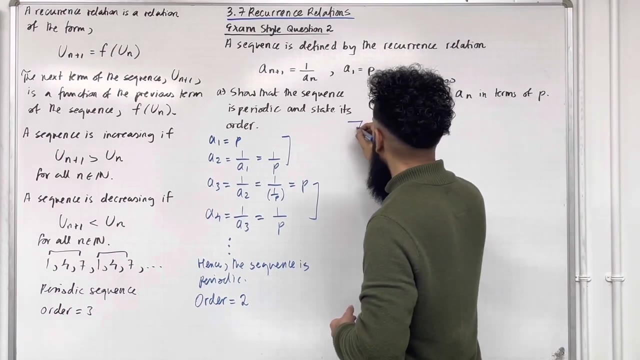 because we've got repetition in 2s. So order is equal to. Let's have a look at part b. Find the sum from n equal 1 to 1000 of a n in terms of p. So, ladies and gents, we're going to start by opening up the sum. So we've got the sum from n equal 1. 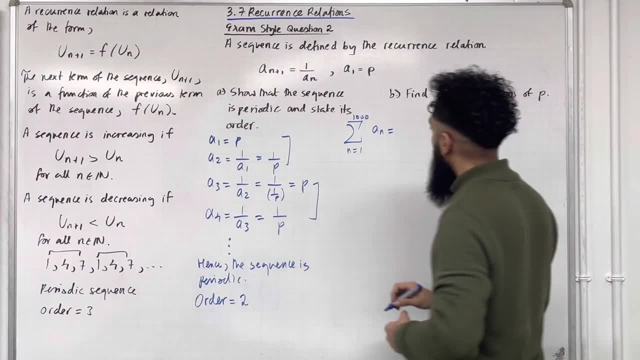 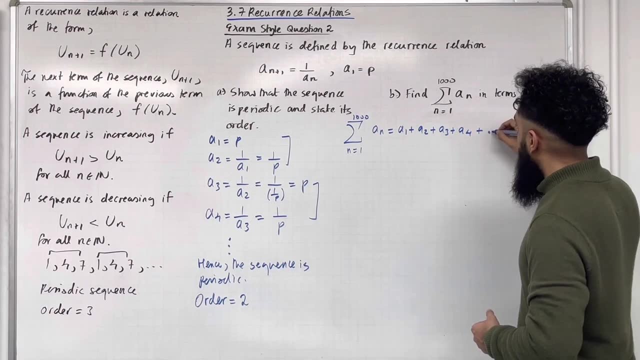 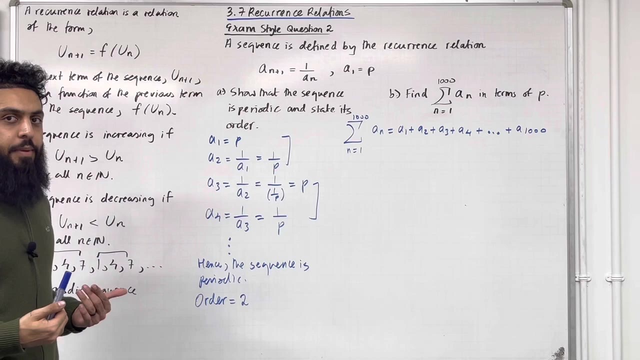 to 1000 of a n. This is equal to a1 plus a2 plus a3 plus a4, plus dot dot, dot plus a1 thousand. Now let's take a step back and see what happens to a n as n changes. So a n is equal to: 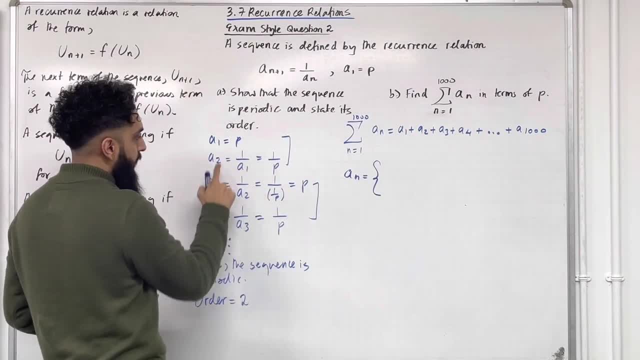 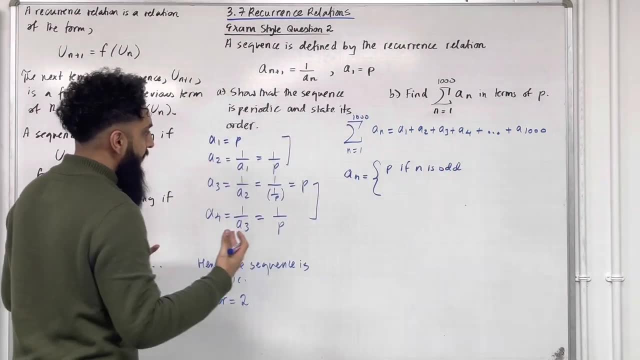 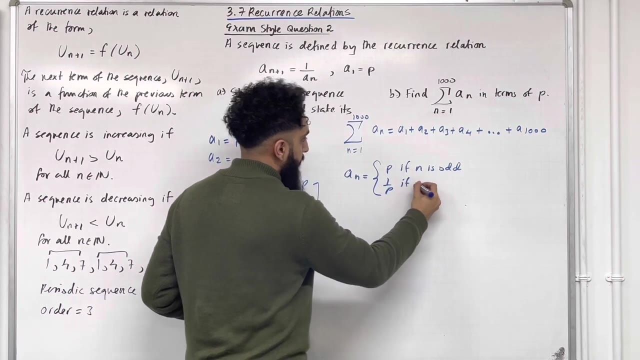 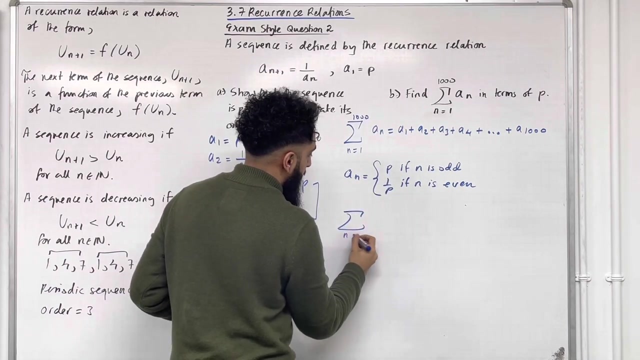 p if your n is odd. So we've got p. if n is odd, a n is equal to 1 over p when n is even So 1 over p. if n is even So, I can go back to this summation. I've got the sum from n equal 1 to 1000 of a n, which is equal to. 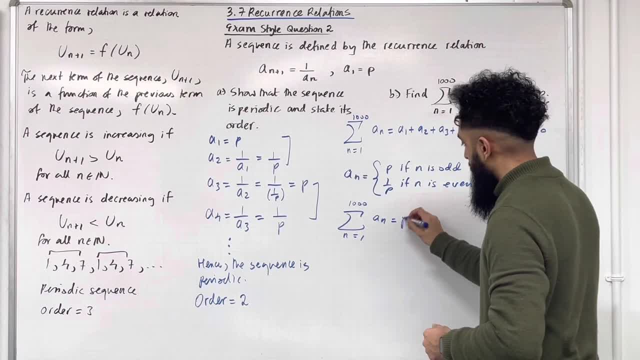 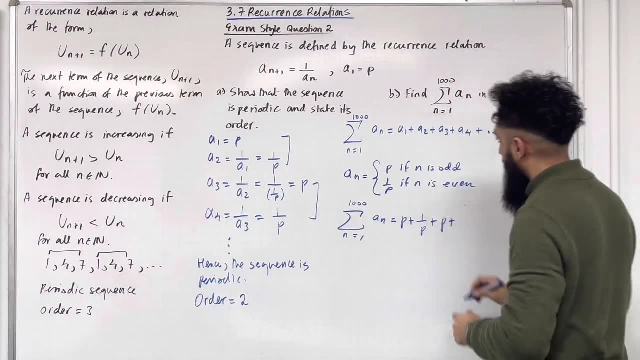 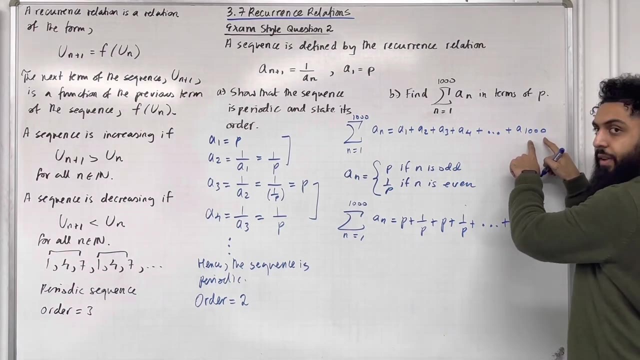 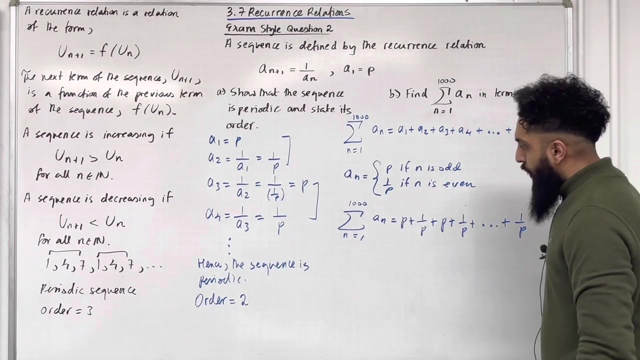 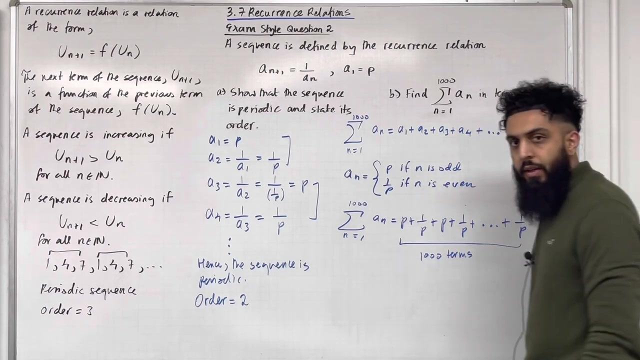 that there's p plus 1 over p plus p plus 1 over p plus dot, dot, dot plus. Now over here the index is even. 1000 is an even number, So that must be 1 over p. Okay, now we're looking at 1000 terms, So we can take 1000 and divide it by the order of the. 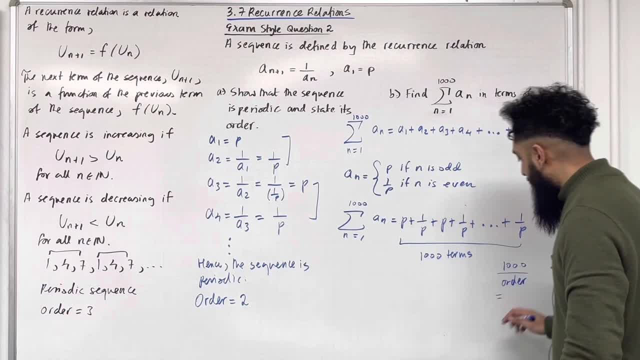 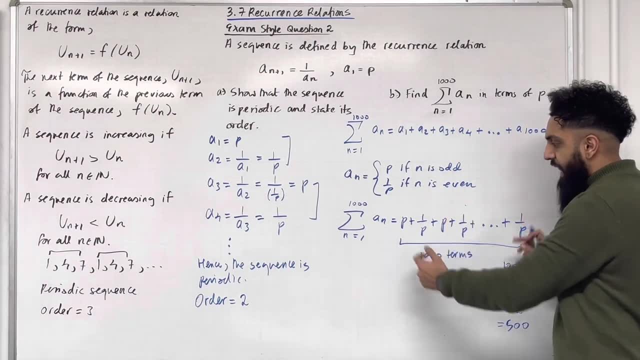 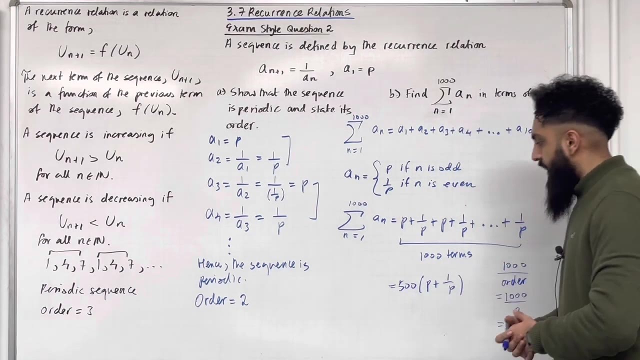 sequence, The order is 2.. So we've got 1000 divided by 2, which is 500.. So, ladies and gents, this sum over here simplifies to 500 lots. So we've got a sequence of p plus 1 over p inside the bracket. And that there, ladies and gents. 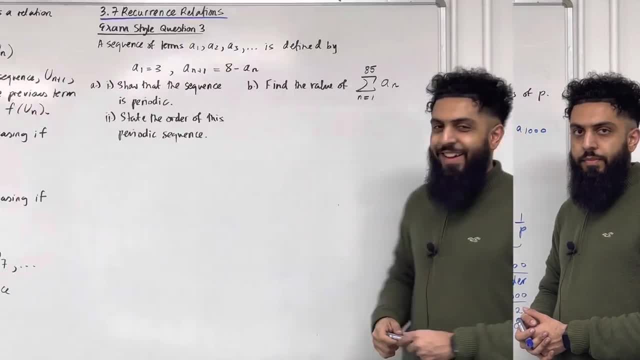 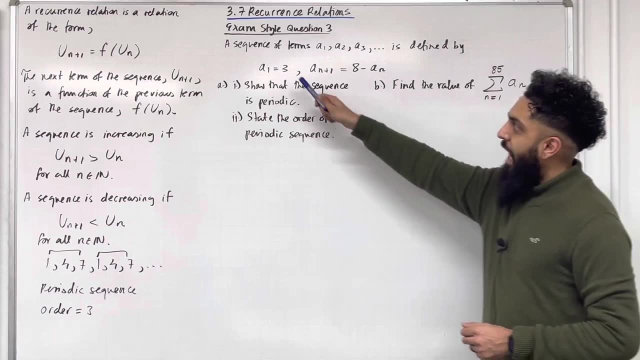 completes part b and exam style: your question 2.. Let's have a look at exam style: your question 3.. A sequence of terms- a1, a2, a3, dot dot dot- is defined by: a1 is equal 3 a n plus 1 is equal 8 minus a n. 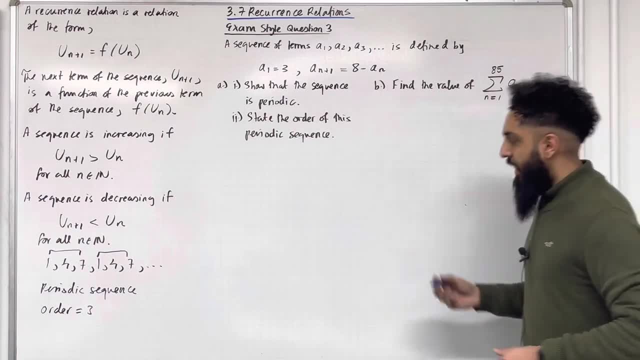 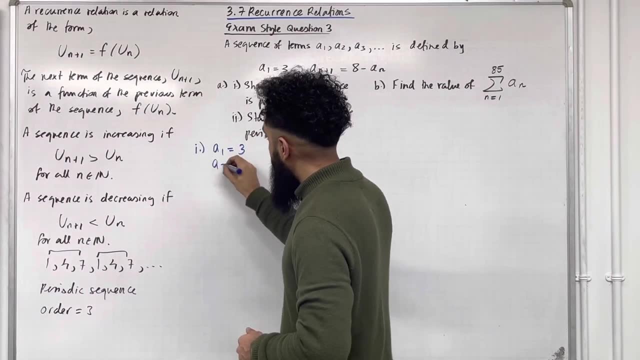 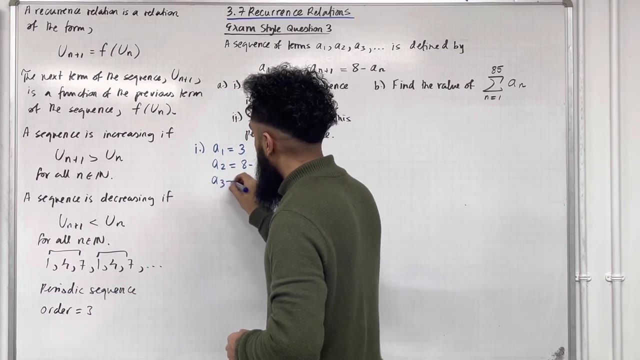 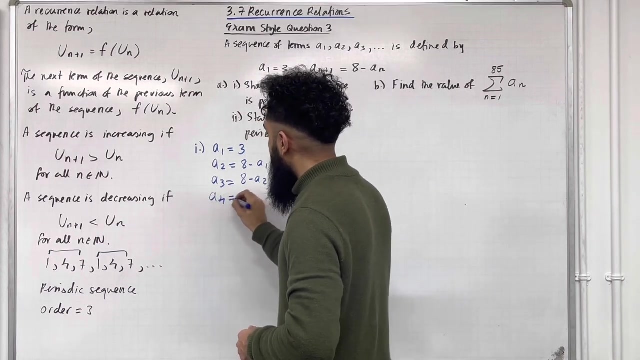 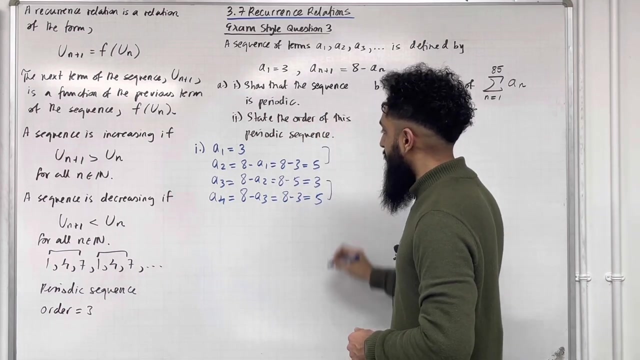 Part a, part 1, show that the sequence is periodic. So let's have a look at part 1.. Firstly, we know that a1 is equal 3.. a2 is equal 8 minus a1. So this is equal 8 minus 3, which is 5.. a3 is equal 8 minus a2.. This is equal 8 minus 5, which is 3.. a4 is equal 8 minus a3. This is equal 8 minus 3, which is 5.. We have repetitions in cycles of 2, dot, dot dot. Hence the sequence. 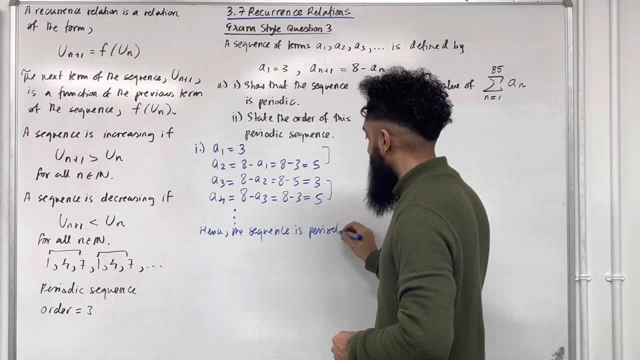 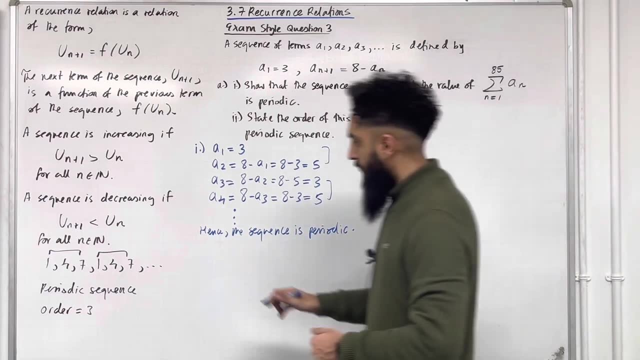 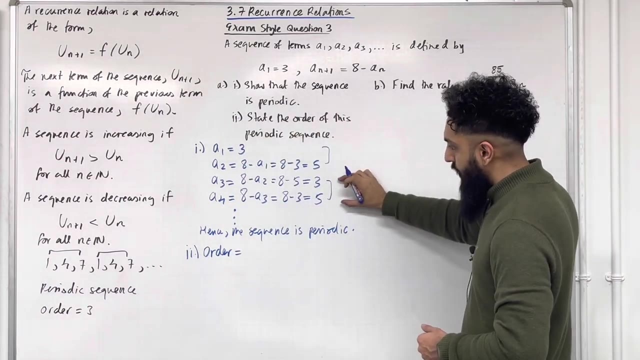 A1 is periodic. Let's have a look at part 2. State the order of this periodic sequence. So we've got part 2. Order equal. Since we have a repetition in cycles of 2, the order is equal 2.. 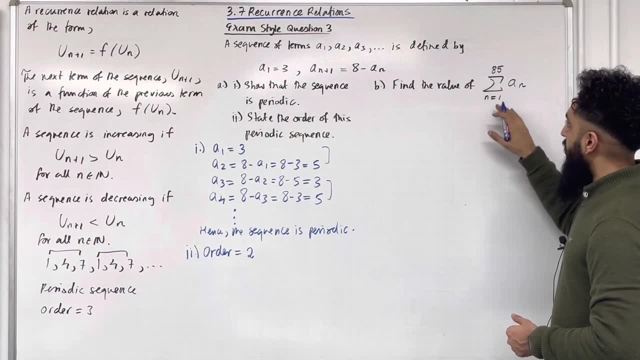 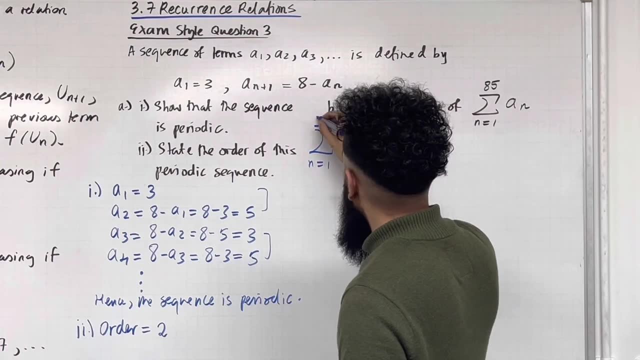 Moving on to part b, Find the value of the sum from n equal 1 to 85 of a n. So we've got the sum from n equal 1 to 85 of a n. Ladies and gents, we can open up this sum. 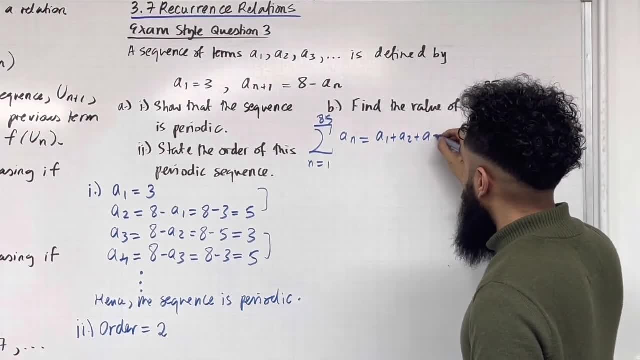 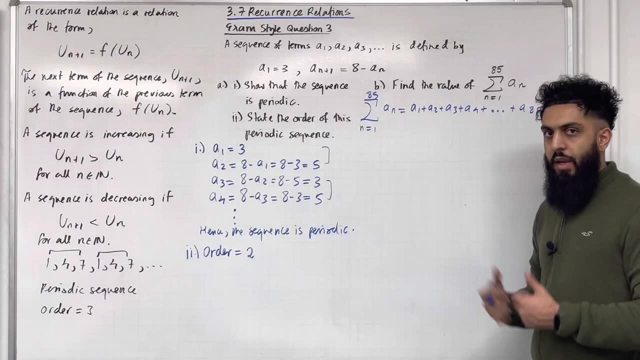 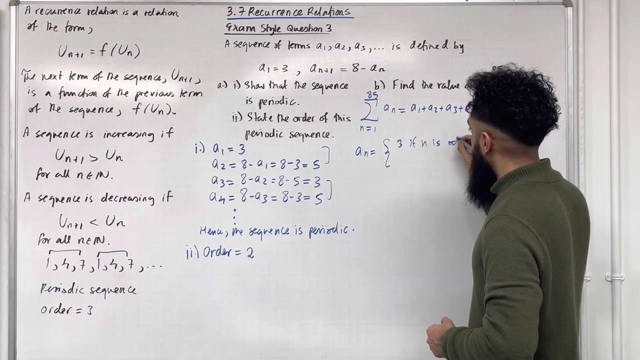 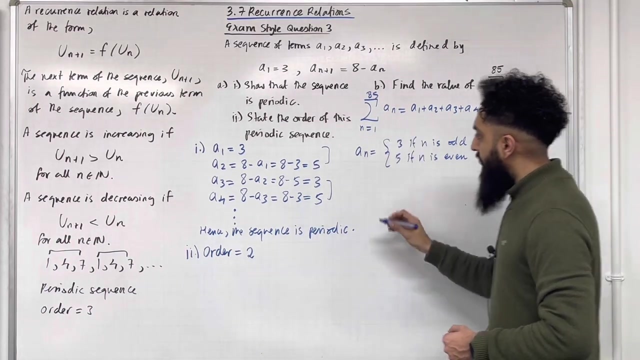 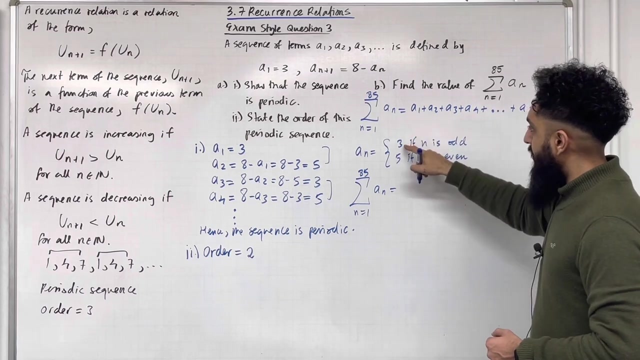 So we have a1 plus a2, plus a3 plus a4, plus dot dot dot plus a85. Now a n is equal 3 if n is odd, It is equal 5 if n is even. So this sum over here, the sum from n equal 1 to 85 of a n is equal a1 is 3. 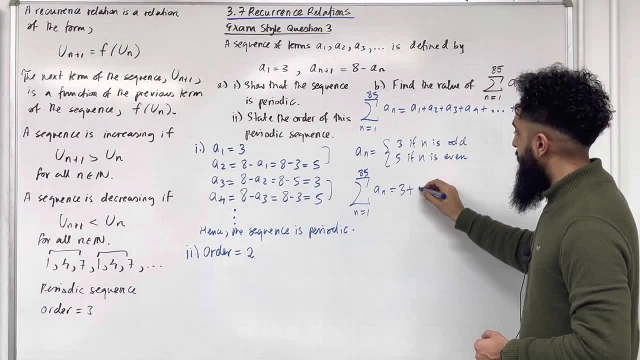 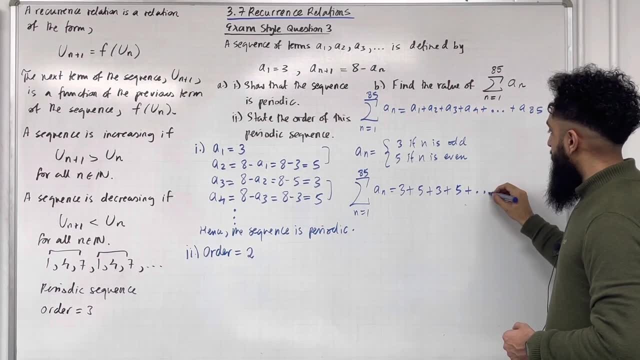 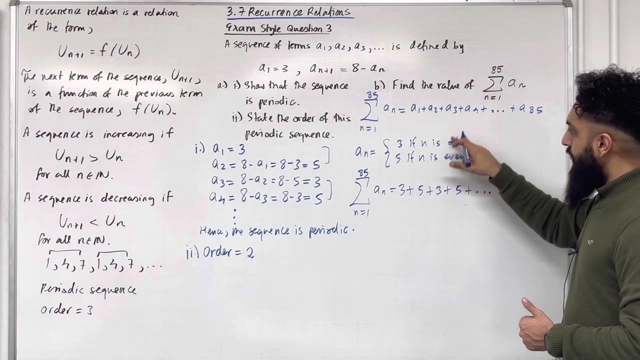 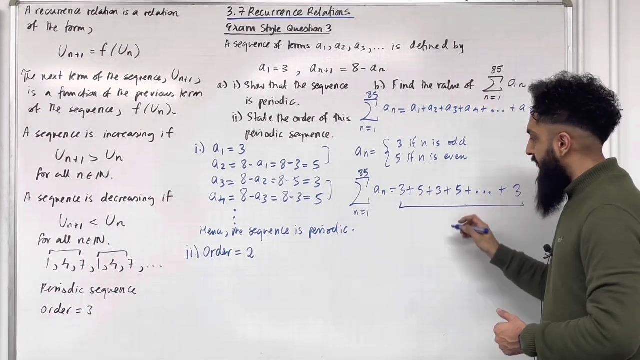 plus a2 is 5 plus a3 is 3 plus a4 is 5 plus dot dot dot plus a85.. Now the index over here, 85, is odd. So if n is odd, we have 3.. Okay, now in this series we have 85 terms. 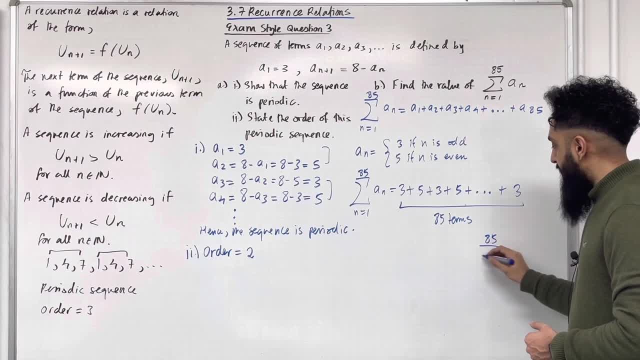 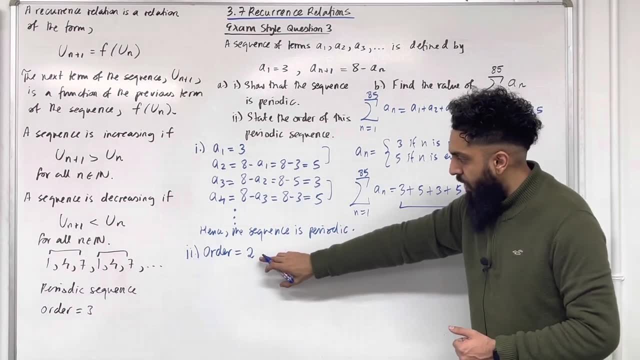 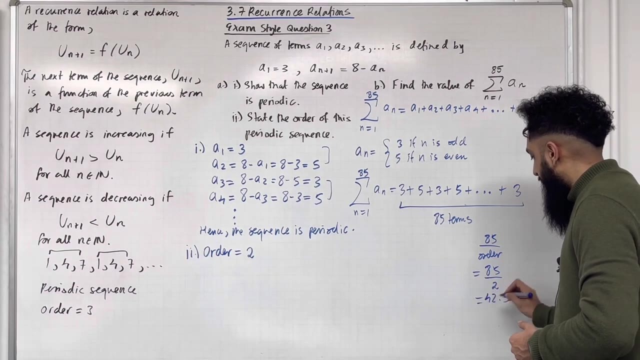 Ladies and gents, we can take 85 and divide it by the order of the periodic sequence. So we've got 85 divided by the order of the periodic sequence is 2.. So 85 divided by 2, 42., 42.5.. Okay, so we're going to round down. So if we round down, 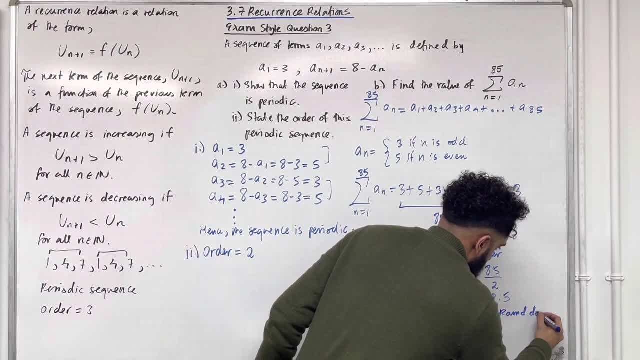 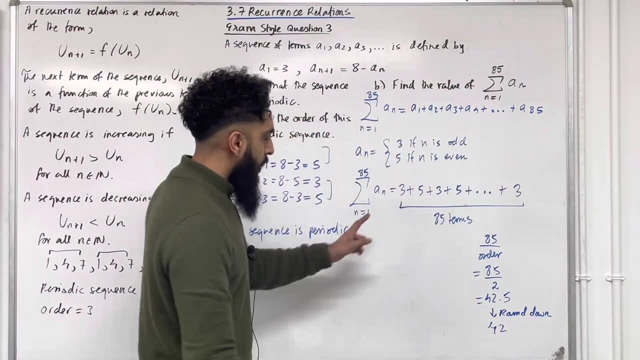 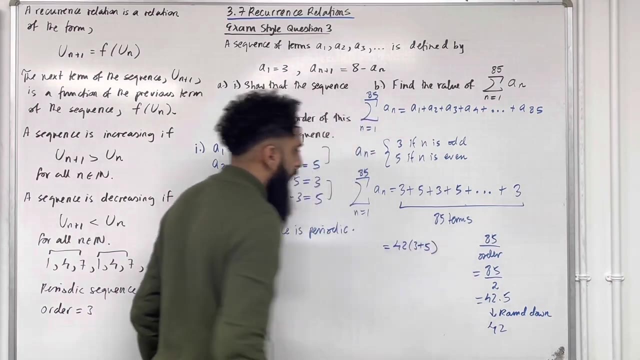 so that we don't miss a term. we're going to round down, we get 42.. So this summation over here simplifies to 42: lots of 3 plus 5.. But we still have that one term, that final term, which is 3.. 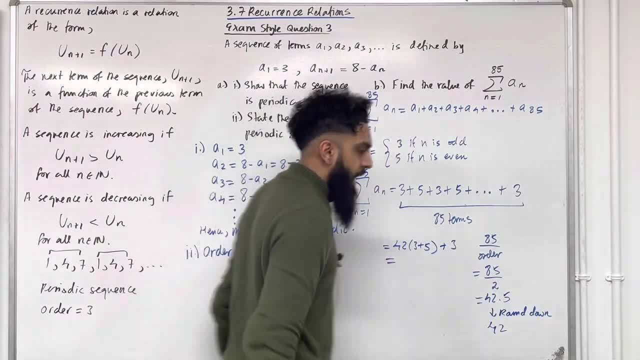 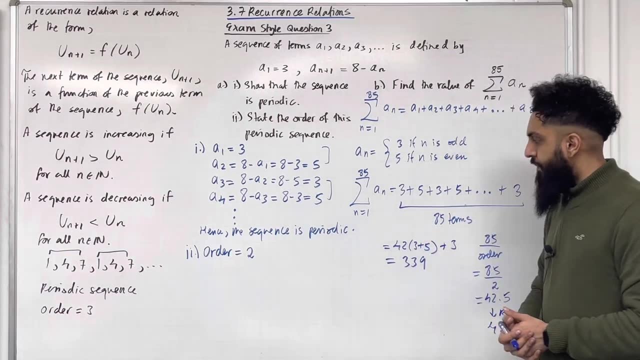 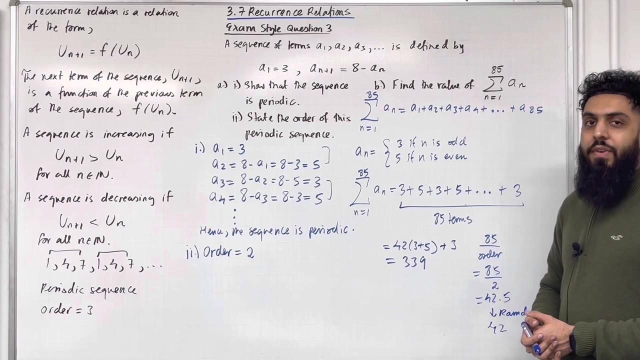 So plus 3.. We can now put this into our calculator And so if we put this into our calculator, we get 339.. This year completes part B of the question and exams. that your question three. If you found this video useful, please don't forget to subscribe. leave a like. leave a comment.